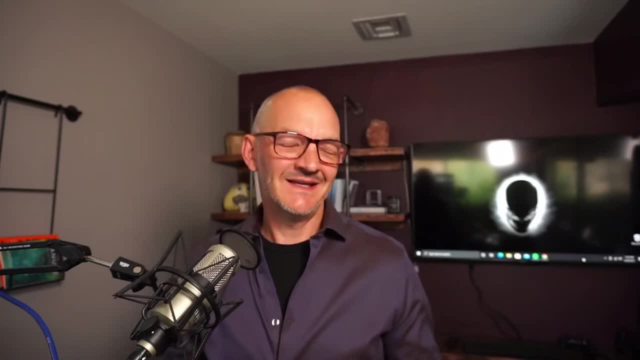 you're saying: well, you can just use async await, and I can, but really async await is just a wrapper around a promise and a promise is just a wrapper around a callback and callback is really just kind of an indicator that I've used the wrong tool for the job. I get it like on the front end. 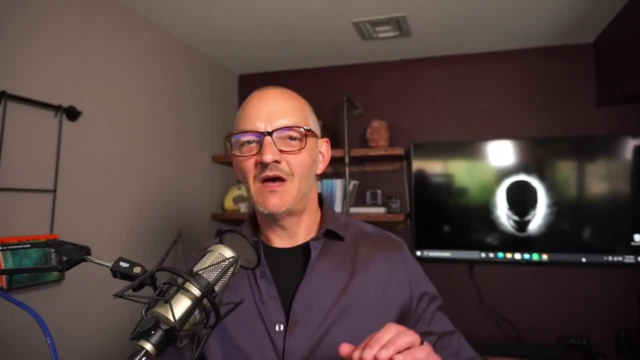 right on the front end, javascript makes perfect sense. things happen in browser land that I can't control and I've just got to wait for them to come back. so it makes perfect sense to have an async tool there. but on the back end I write my code very structured. everything is very organized, very 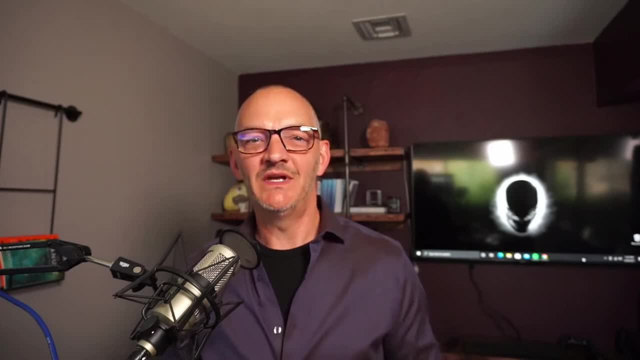 methodical. I know exactly what order I want things to happen in and when I want them to happen, and what I want to happen in and what I want to happen in and what I want to happen in and what I want to happen after that happens. and to me just doing all of this async await callback. I promise you. stuff is just added complexity that doesn't need to be there. whenever I talk about this with people, the other thing I get is: oh, but using nodejs means I can use javascript on the front end and the back end? yes, it does, but if the ability to learn multiple languages 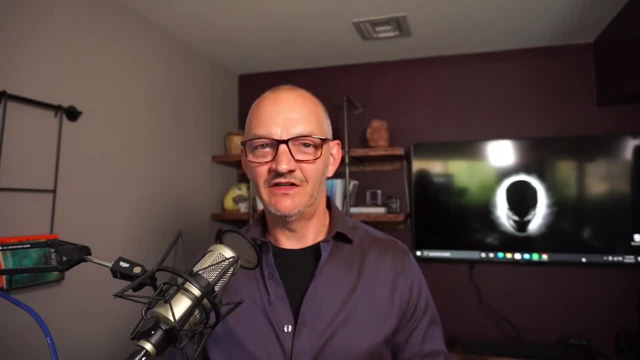 is your sticking point and your limitation as a developer. you're really, really going to struggle throughout your career. all right, case in point: go back. if you haven't watched my geo routing video, I'll put a link to it up here. case in point: there the problem. 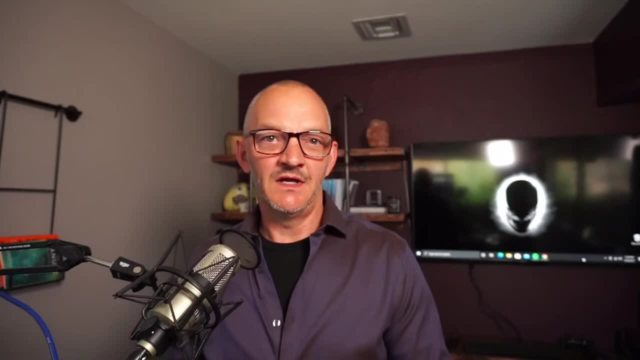 there was in a sequel query and they weren't writing sequel code, they were letting an ORM do that for them. and so that's kind of the problem, right, because you can't just know one language and be a successful developer, you've got to know javascript if you're doing front end work, html, css on the back end, whatever back end language you use. 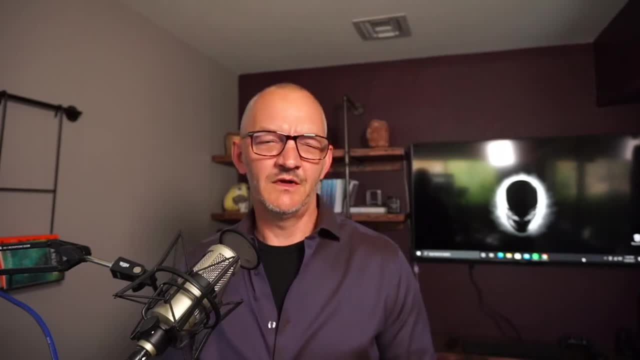 let's still assume that you're going to use nodejs, so you get javascript there as well. but you also have to know sequel right, because you're writing database queries. you have to be able to understand that that's the right query to use or how to optimize it when it's not correct. 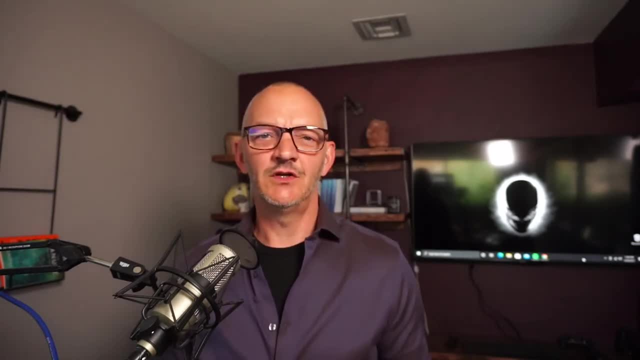 you're also involved in the deployment of your application, which ultimately, no matter what solution you use, is going to involve some level of bash scripting. so you've got to know bash and over time, javascript itself is going to change to where it no longer resembles the javascript that you're writing today, or something else is going to come along and take its place, and you're going to have to learn that. so this whole single language thing is just. it's not practical. there's not a scenario that I can imagine where you're going to be able to write javascript and just javascript, as you write javascript today, for the next 20 years in your career. 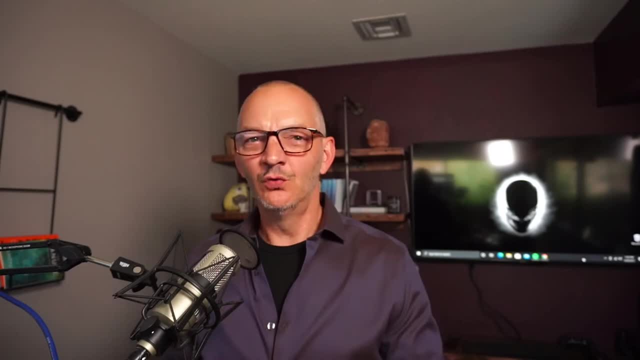 so it doesn't make sense to me to pick the wrong tool for the job for the sake of, for the sake of an excuse. it's not even a valid excuse. so I get that. that's not the most popular opinion in the world. as a matter of fact, I think I'm probably one of the few people that have that. 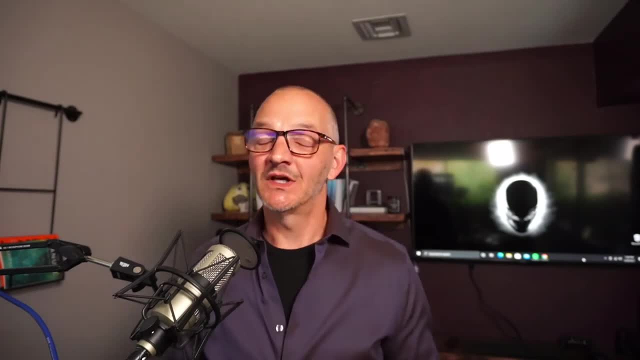 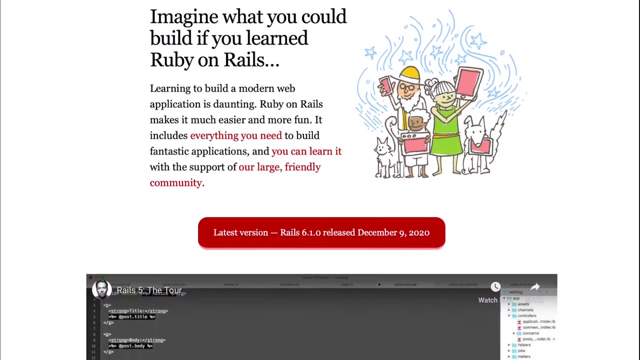 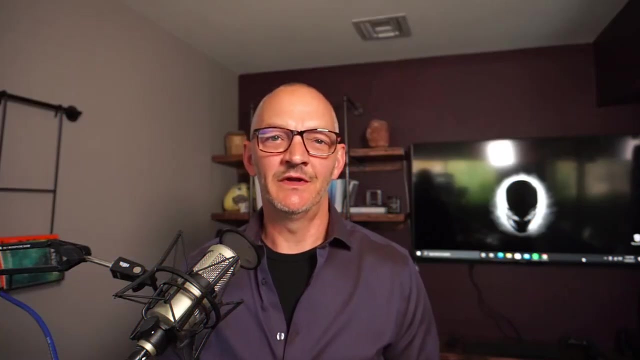 opinion, but I really do believe I'm right on that. when it comes to picking a back-end language, though, here are the ones that I do think are good. fits ruby on rails. it's very, very opinionated, but it works really really well. you can't argue with with that. pythons- another good one. python is super. 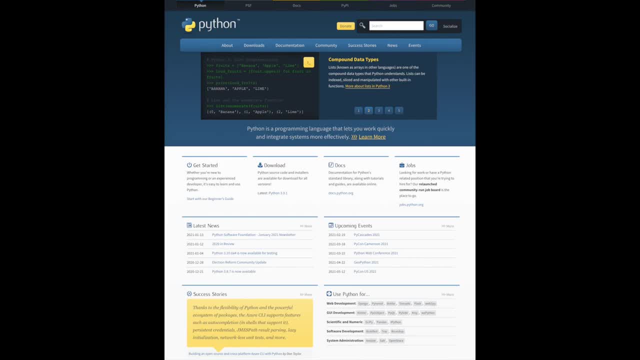 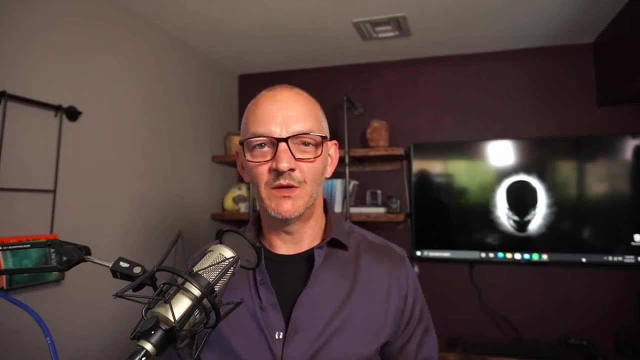 easy to learn. let's make sure we're using python 3 and not python 2. it's time to let it rest in peace. but there's a ton of support for python, python based applications and python web servers and lots of tools to make that easier. the one that I'm really excited about recently is go. 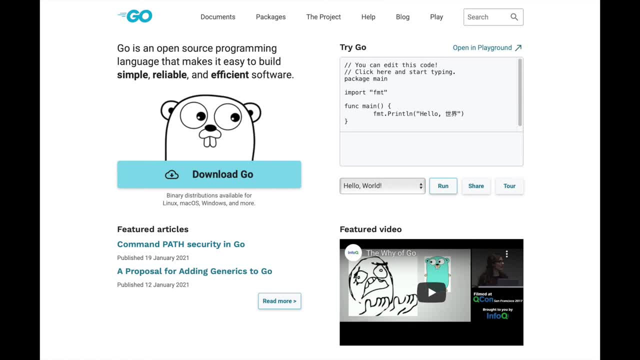 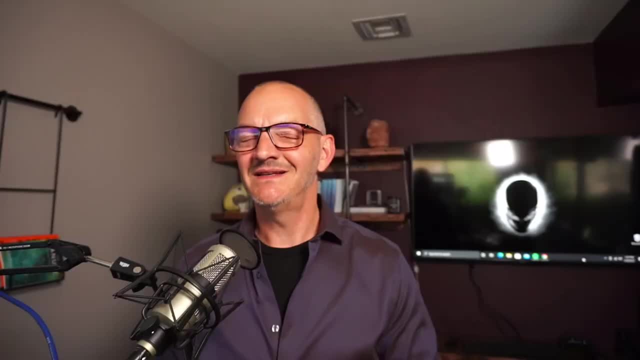 and the reason I like go is because it's a tight language. it's a little more difficult- at least it was a little more difficult for me to learn, but I really liked it once I got the hang of it. the big things I like about it is that testing is built into it. testing go code is 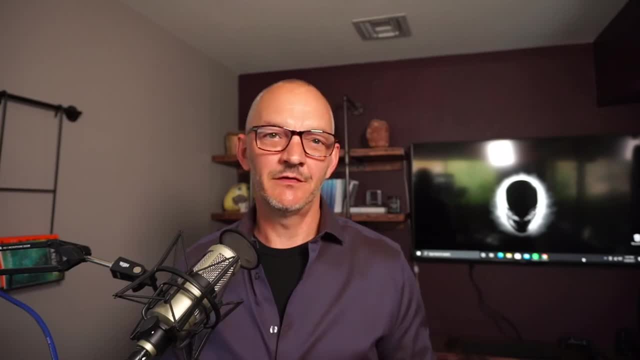 native to the go framework itself. you don't have to go find some third-party test application to write tests for it. and the other thing is it's got built-in performance measurements as well, so you can do performance testing against your code from right within the go language itself. and again,